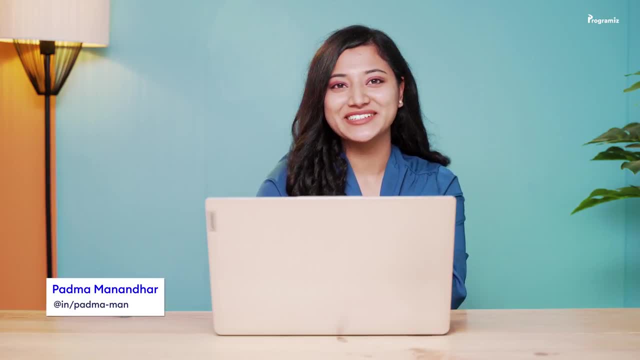 Hey guys, this is me, Padma from Programmees, and welcome back to this series on C-Programming. In this video, we'll learn about if-else statement. in C-Programming, We'll learn to create decision-making programs that perform one set of tasks under a certain condition. 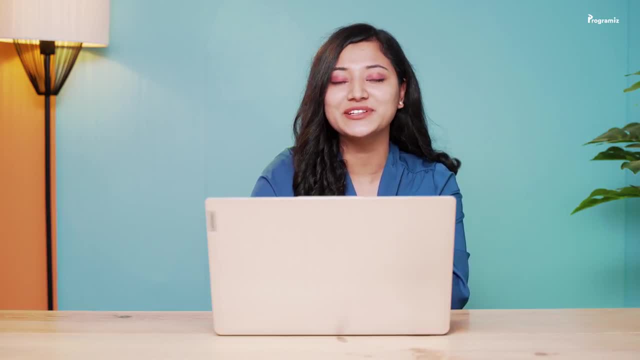 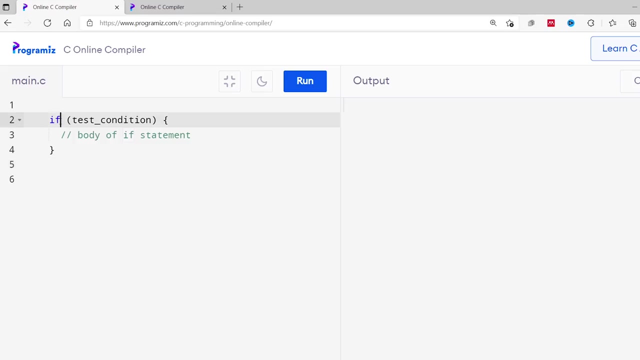 and another set of tasks under different condition. So let's get started. In C-Programming, we use the if statement to create programs that can make decision. Let's start by looking at the syntax of the if statement. The if statement starts with if keyword and. 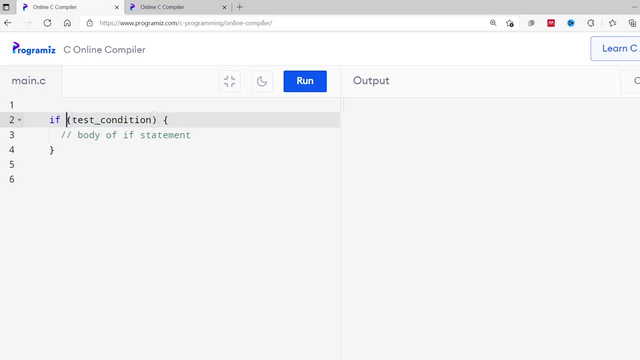 is followed by the test condition inside the parenthesis. This test condition is a Boolean expression that results in either true or false. If the test condition is true, the body of if statement is executed. Otherwise, it is skipped from the execution. Now that 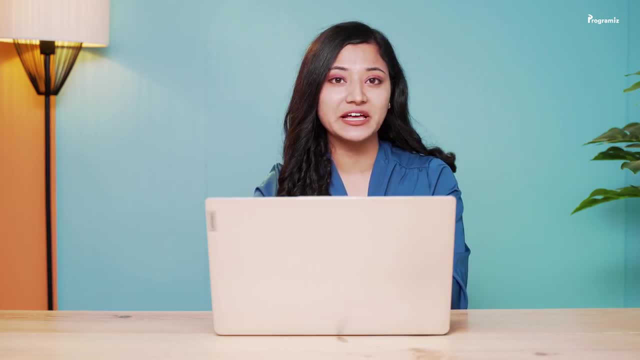 you know the syntax of if statement. Let's try a working example. Suppose there is an election going on and to cast the vote, your is must be 18 or more. If your is is 18 or more, we'll print you are eligible to vote. 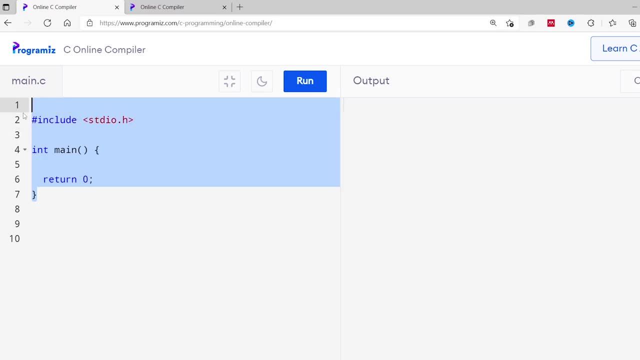 Let's see how we can implement this Here. I have a basic C-Program. Now I'll create a variable to store is- int is. Now I'll ask the user to input their is. For that I'll use printf statement and print the message. 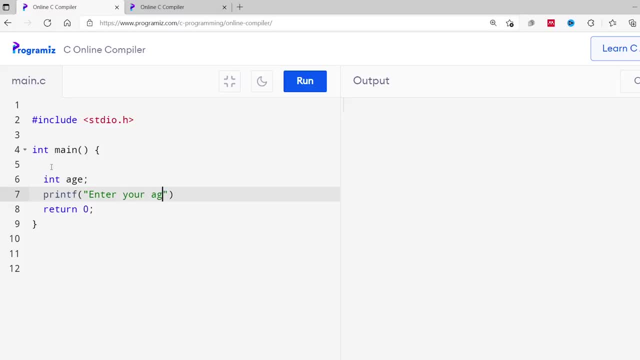 This is like: enter your is, Then I'll use scanf statement to take the input percent D comma ampersand is. Then I'll use if condition to check if is is greater than or equals to 18.. If this condition is true, I'll print you are eligible to vote. 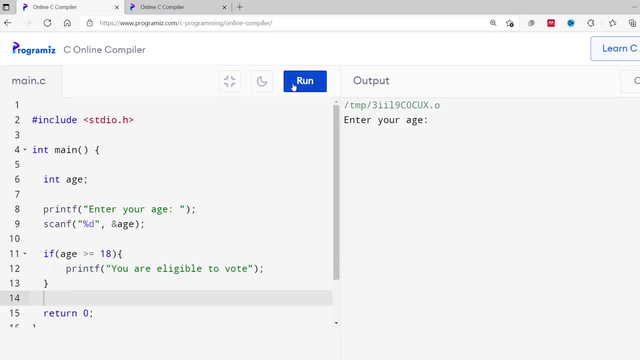 Now let me run this program Here. I'll provide 31 as the age and I'll press enter. As you can see, you are eligible to vote is printed Here. the value is 31,. so our test condition is greater than or equals to, 18 is true. 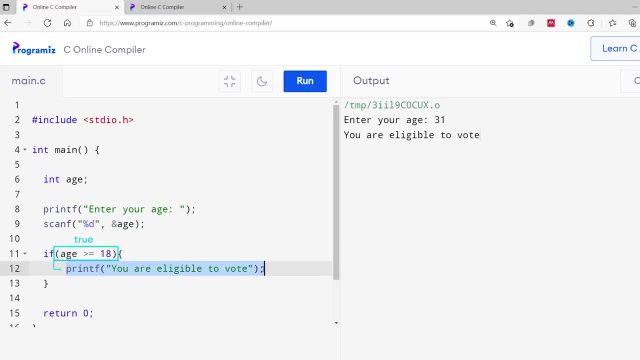 That is why this print statement is executed. Now let me run this program again. This time, instead of 31,, I'll enter 15. This time, nothing is printed on the screen. This is because the age is 15, so the test condition age is greater than or equals to, 18 is false. 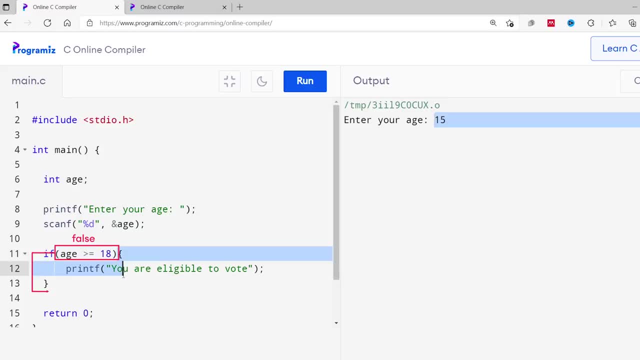 So the body of the if statement: Our program is working fine, but it is not printing anything when the age is less than 18.. We might want to print something like: sorry, you are not eligible to vote when age is less than 18.. 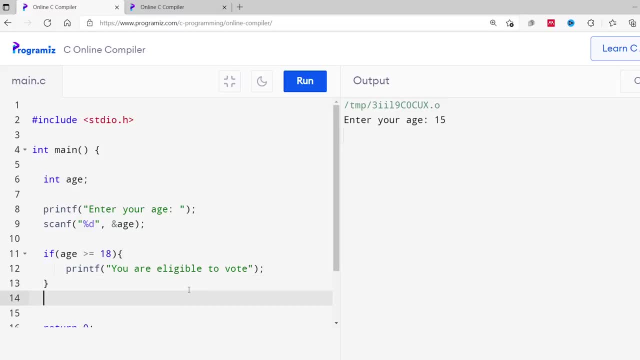 So I'll add another if statement. So I'll say: if age is less than 18, I'll print: sorry, You are not eligible to vote. Now I'll run this code and I'll enter 15 again. Here you can see: sorry, you are not eligible to vote. is printed. 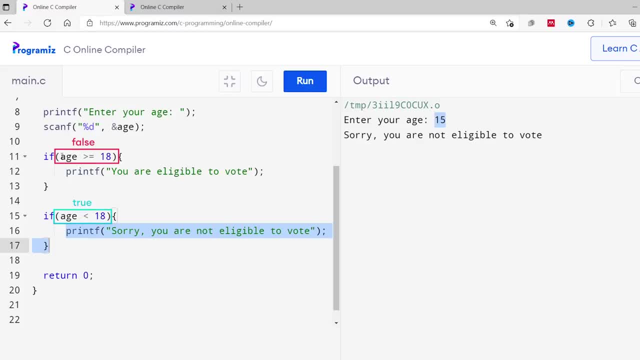 This is because age is 15.. So this condition- age is greater than or equals to 18- is false. Therefore this statement is skipped. However, this condition- age is less than 18- is true, So this statement is executed. 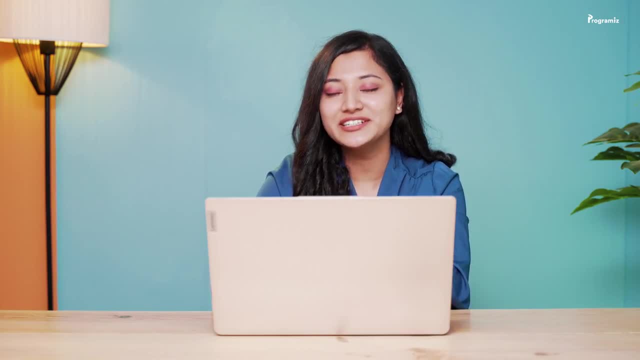 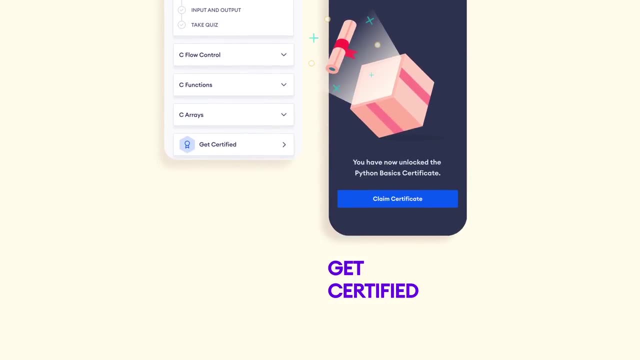 By the way, if you're watching this, there is a good chance. you want to improve your skill in C programming. Lucky for you, we have a mobile app that provides a well-structured C programming course with certification at the end, And you can use the app, alongside the video, to practice on the built-in compiler. 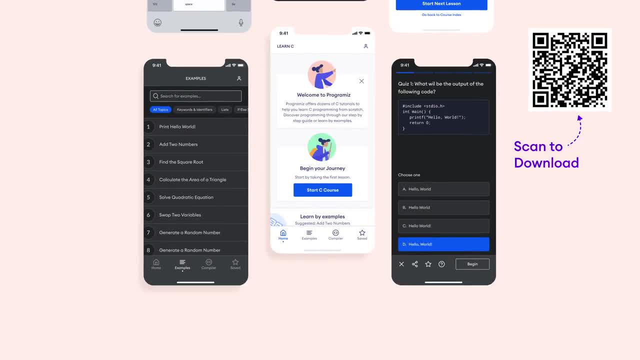 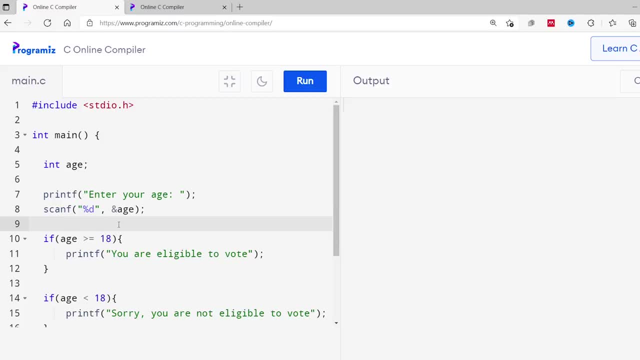 Our course is free, So download now by scanning this QR code or click the link in the video description. I have this code from the last segment. I'll remove this code to get the user input And I'll manually assign the value of age equals to 15, so that it's easier to focus on the logic of the if statement. 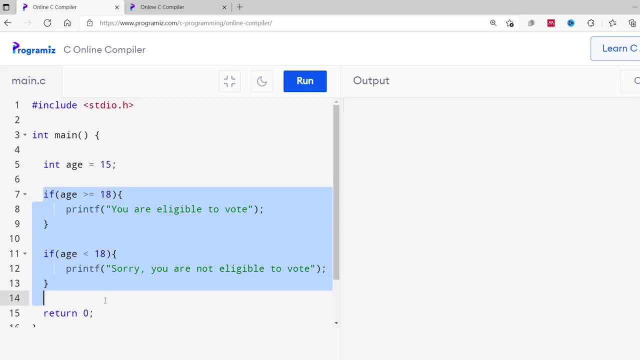 In this program, I have used two if statement to perform two different tags. We know that the person is eligible to vote only if the age is greater than or equals to 18. And if the condition Is not met, we know that the person is not eligible to vote. 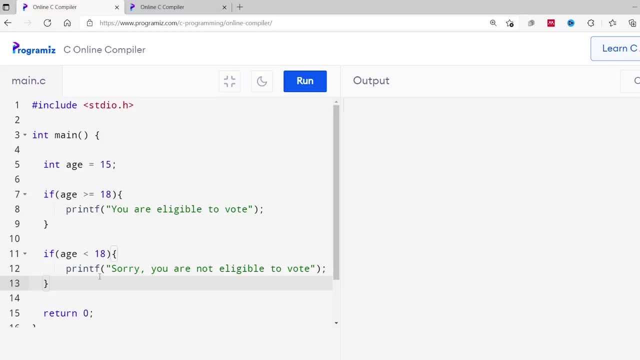 In such cases, instead of writing the second if statement with the condition we can use else clause, Let's first look at the syntax of the if statement. with the else clause On your screen, you can see how it looks. So what happens here is, if our test condition is true, statement inside the body of if statement is executed. 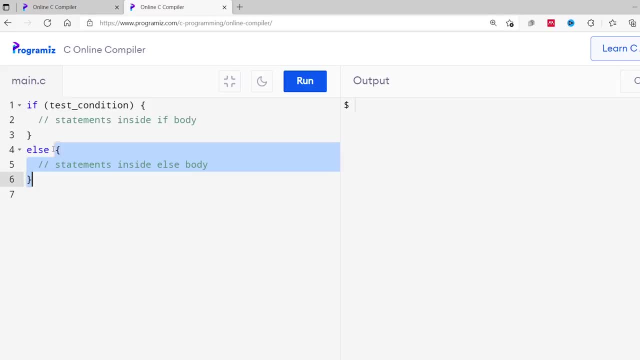 And if it is false, statements inside the body of else are executed. Now, getting back to our code, to check if the person is eligible to vote or not In this program, I'll use the else clause instead of this second if statement. 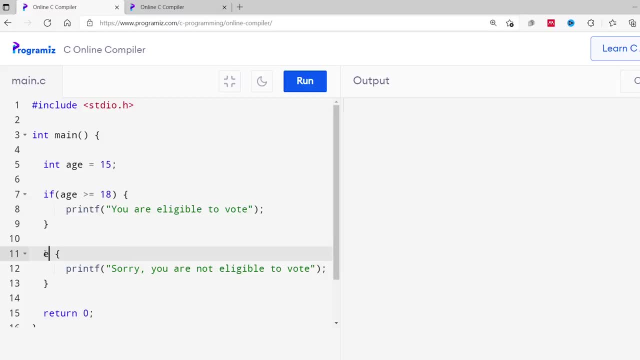 So I'll remove the second if statement and replace it with else. Now let me read this code in plain English: Age is greater than or equals to 18.. Then print your eligible to vote. Else print. sorry, you are not eligible to vote. 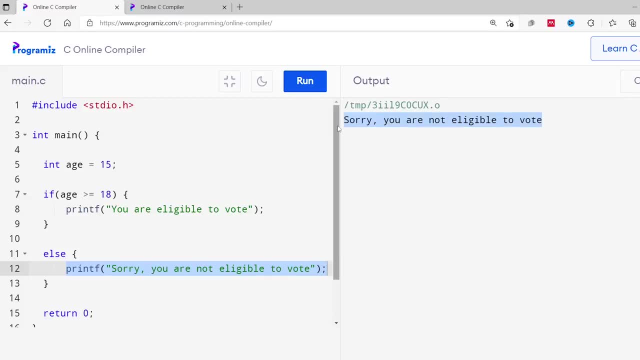 Now, when I run this code, you can see: sorry, you are not eligible to vote is printed. This is because age is 15, which is not greater than or equals to 18.. So we get the output: Sorry, you are not eligible to vote. 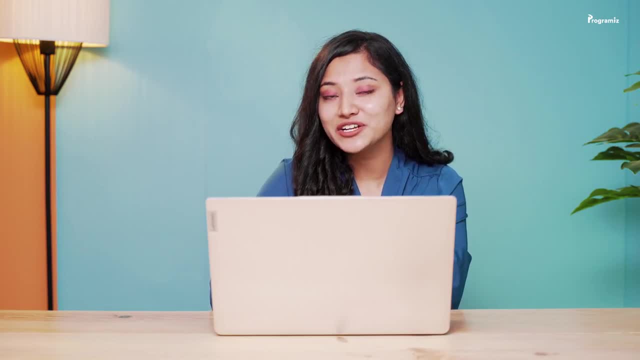 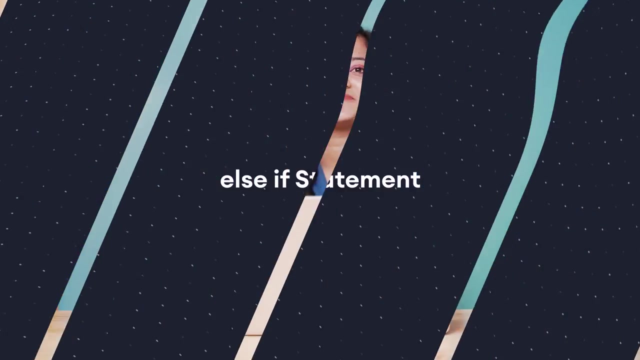 Okay, guys, we need your support to keep these types of content free for all users. YouTube really likes engagement on the video, So leave a comment below, Press that like button, hit subscribe if you haven't already. Let's get the engagement score higher so that more people can discover and enjoy these courses. 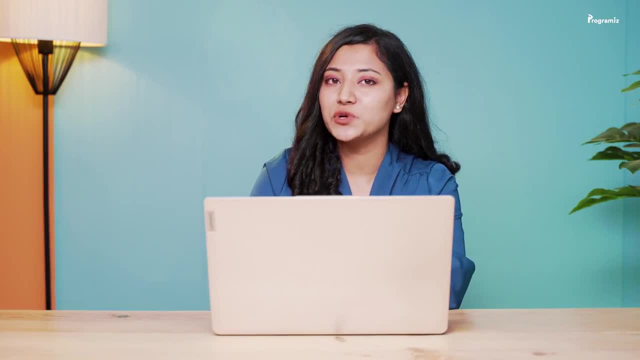 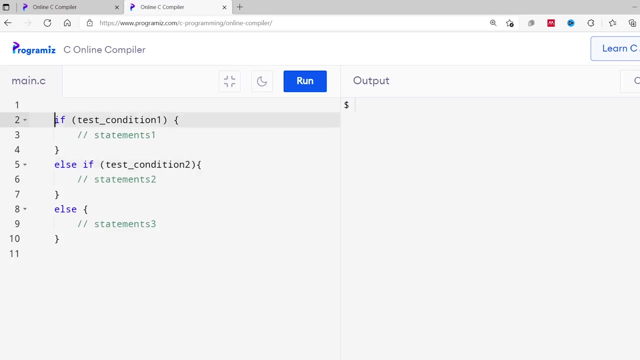 The if statement with else clause allow us to make a choice from two different options. However, sometimes we need to make choice from more than two options. In those case we can use else if clause with test condition. Let's see the syntax first. 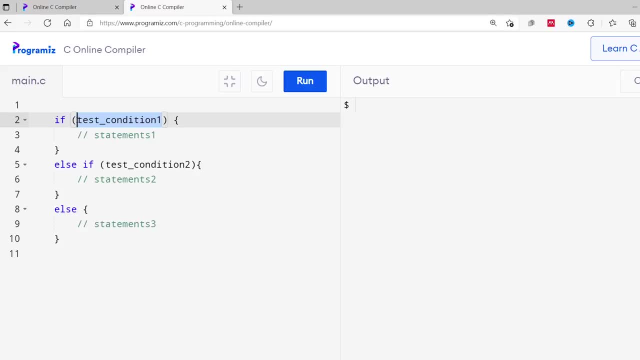 The if statement Checks the first condition inside the if statement. If it is true, the body of if is executed and the statement two and the statement three are skipped. However, if the first test condition is false, the control of the program jumps to the second. 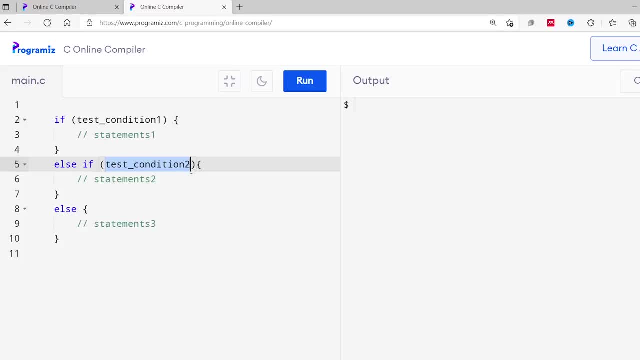 test condition. If this condition is true, the body of the else if statement is executed and other statement are skipped. If both the test condition One and the test condition two are false, then only the else body is executed. If necessary, we can add as many else if clauses as we want for our program to work. 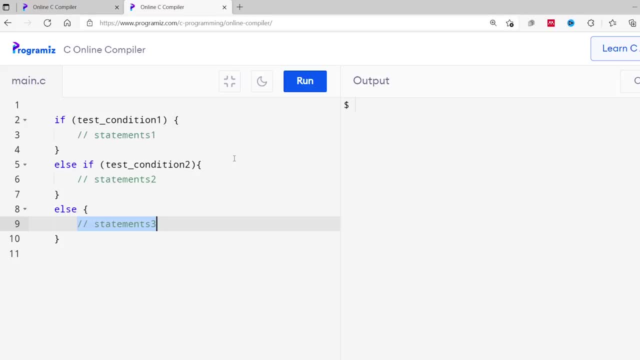 And among all those alternatives, only a single block of code is executed. Now we know how the else if clause works. Let's get back to our code to check whether a person can vote or not. Here, the is variable stores the is of the person. 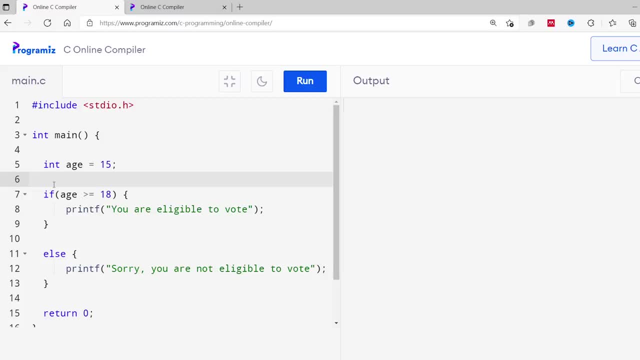 Currently the is of oldest person is 120. So I want this program to consider is greater than 120 as invalid. Similarly, the is cannot be negative, So I also want to mark less than zero as invalid. Now I want to include these two additional condition in our program. for that I'll use 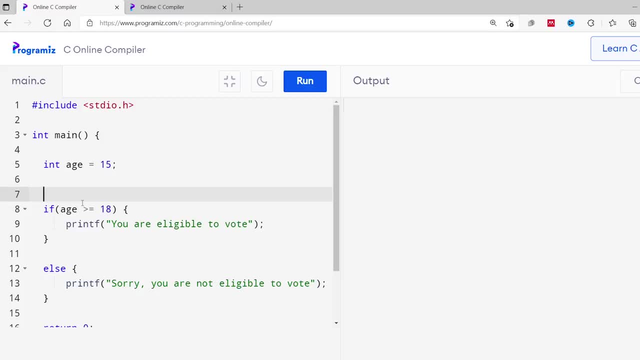 else if clause. Now I'll modify this code So if is is greater than 120.. I'll print invalid is, Invalid is And else if. So if is is less than zero, That is negative value. Then will print Is invalid. 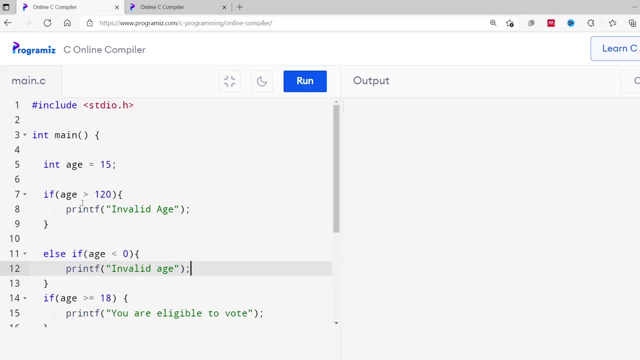 As is. i'll change this if to else. if so, as you can see, i have included one if condition, two else if condition and finally one else condition. here i'll change the value from 15 to 130. now i'll run this code here: the age is greater than 120, so we get invalid is as our. 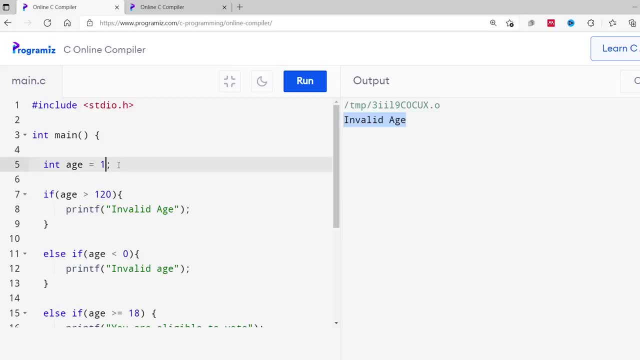 output. now let's change the value of this is from 130 to minus 4 and let's run this again. this time we get invalid is again. so this is the condition of else. if here is is less than 0, so the output we got is invalid ease. now we can add as many else. 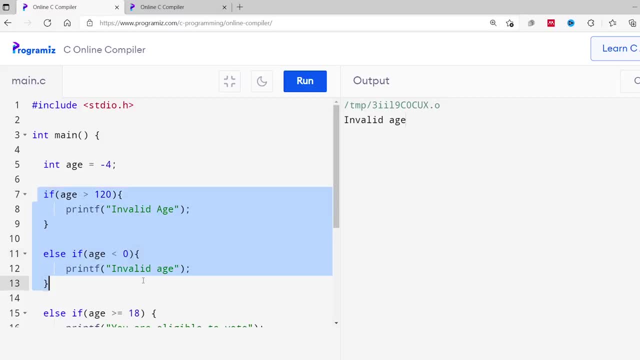 if condition as we want here we can see these two condition are performing the same tax printing, invalid is. in this case we can combine both the condition together using logical operator. here the is is invalid if it is either greater than 1 or 20 or less than 0. or let me modify: 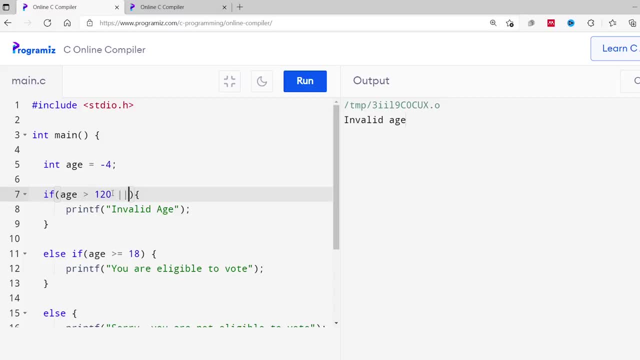 this code, so i'll cut this, i'll use logical or and put here: is less than 0, so i'll change this value from minus 4 to minus 1, and when i run this code i get invalid is as output. now, as long as the. 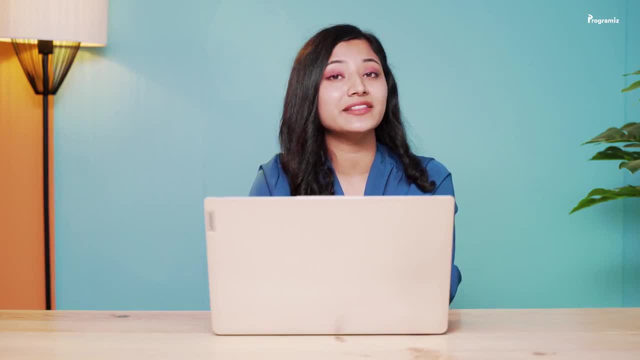 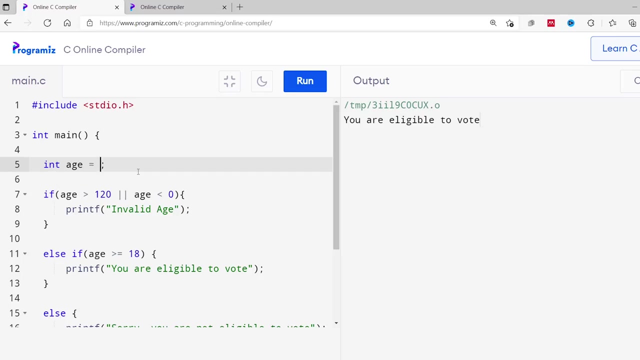 is is an integer number, our program works correctly. and the extra condition: make sure the is is neither greater than 120 or less than 0 and for any other value of is, the program runs as intended. if we provide the is equals to 50, so let's do that. i'll provide the value of is equals. 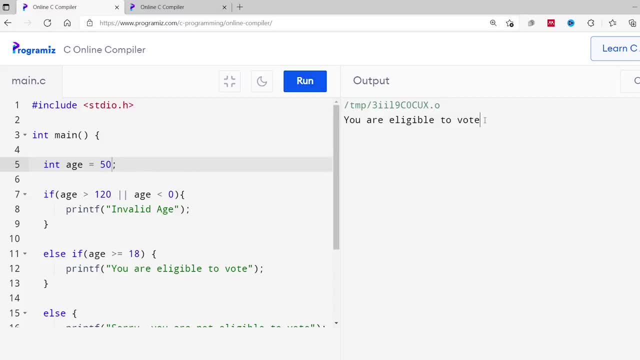 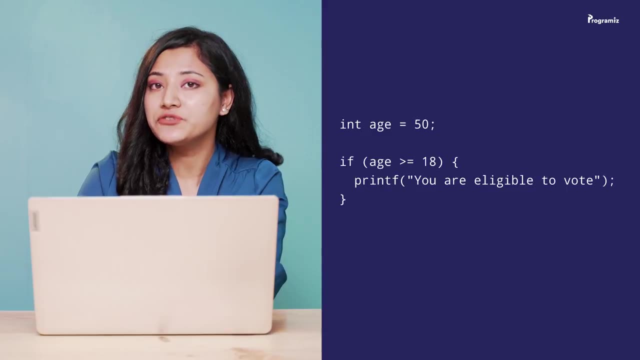 to 50.. 50, i'll run this now. this person is eligible to vote. before we end this video, one quick tip for you. if the body, if else block, has only one statement like this, then we can omit the curly braces of the if block like this. as you can see, the syntax of the if statement is pretty simple. 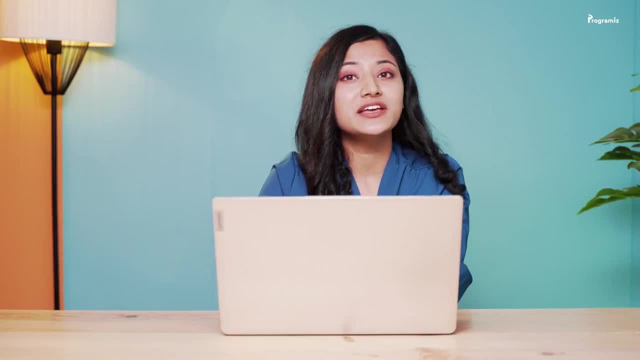 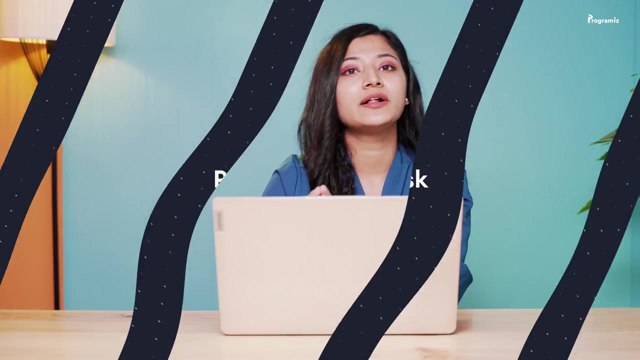 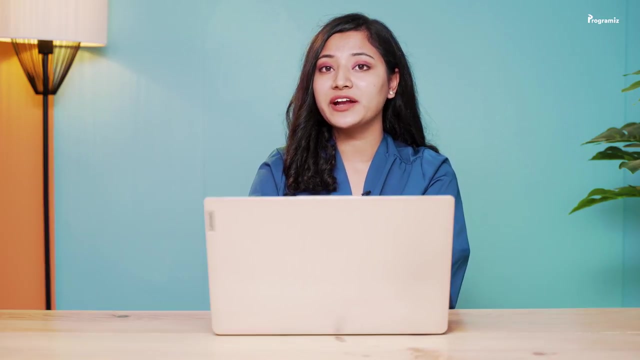 the harder part is the logic behind the test conditions. so you will get better at creating test condition with practice. also, be sure to check our video on the comparison and logical operators that are used to create the test condition. the link will be in the video description below. we have covered a lot in this video. it's time for you to practice what we have. 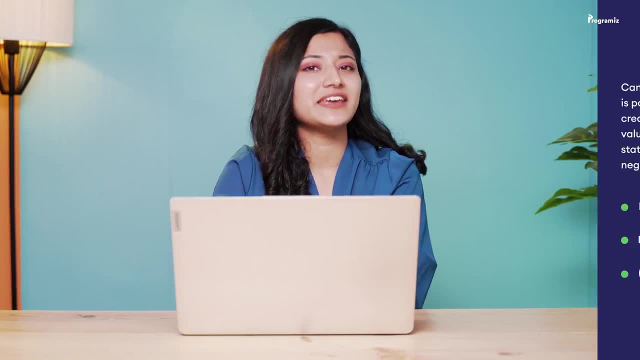 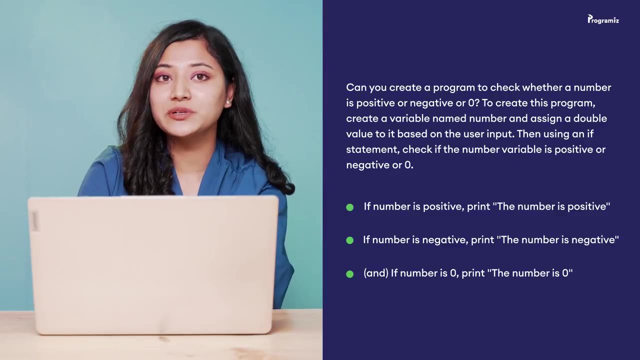 learned. here is one programming challenge for you to solve. can you create a program to check whether a number is positive, negative or zero? to create this program, create a video variable named number and assign a double value to it based on the user input. then using an if. 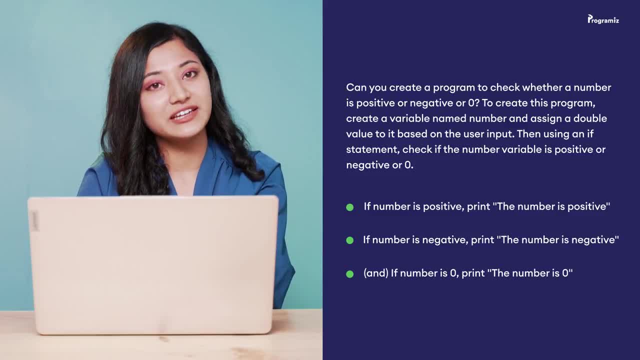 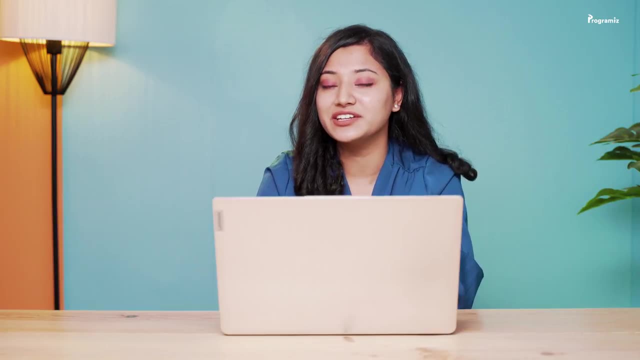 statement: check if the number variable is positive, negative or zero. if the number is positive, print the number is positive. if the number is negative, print the number is negative. and if the number is zero, print the number is zero. you'll find the all the answer to this question in our github.